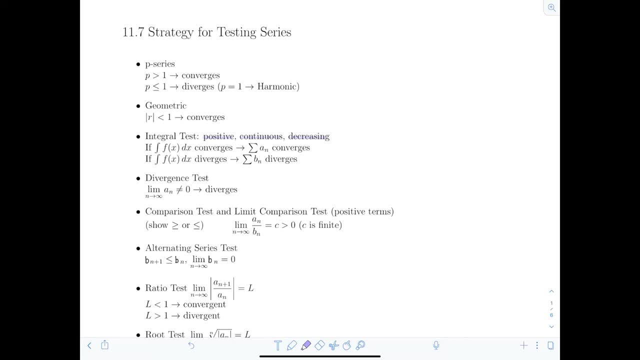 integral of f of x diverges, then the sum of What should be a, n Diverges. Alright, Test for divergence: The limit as n approaches infinity of the terms a, n. if it doesn't equal 0, then we know the series diverges This. 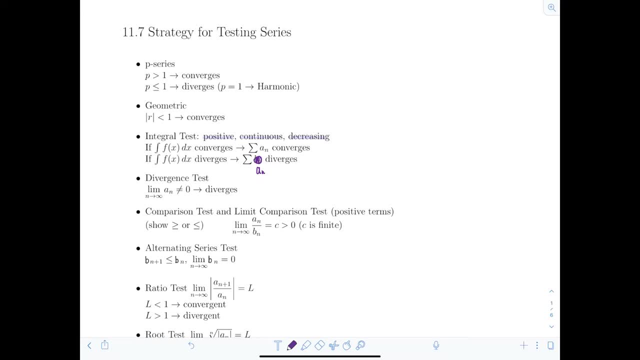 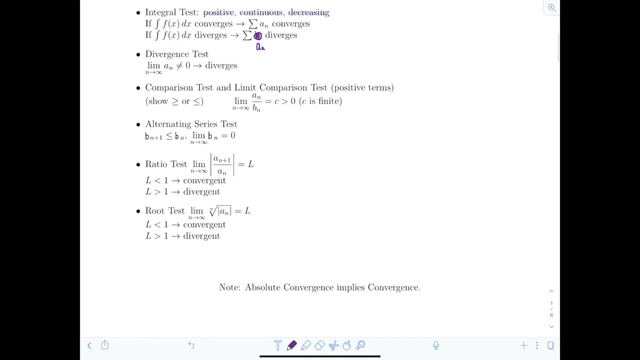 is a good one to just always do in your mind before you even pick another test. to go on with Comparison test and limit comparison test. So for direct comparison test you have to either show that the terms of your series are greater than the terms of another divergent 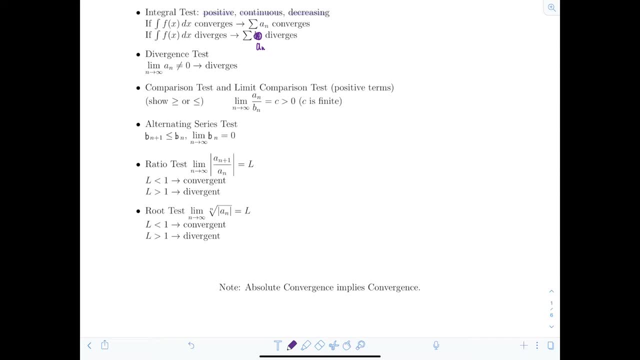 series In order to have a conclusion. Or you need to show that the terms of your series are less than or equal to the terms of a convergent series, So be careful with that. Or if you just do limit comparison, then you need to show that the limit as n approaches infinity. 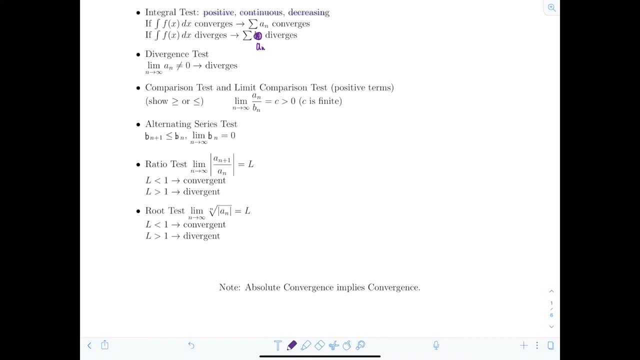 of the ratio of the terms is equal to a constant, Finite constant, not negative, not 0.. Okay, then we have the alternating series test. If the terms remember, b, n is the absolute value of a, n. If they're decreasing and they're decreasing, then we have the alternating series test. 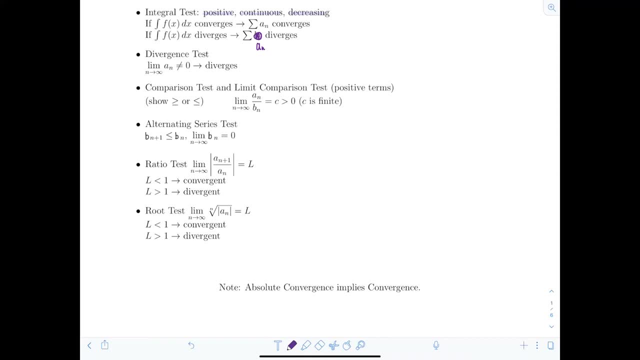 If the terms- remember, b, n is the absolute value of a, n, If they're decreasing, and they're decreasing, then we have the alternating series test. So here we have the alternating series test. If the terms are zero, then we can say that the series converges. Then we also have the 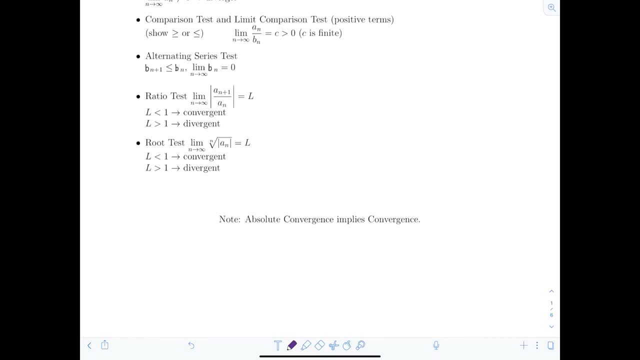 ratio test. So the limit as n approaches infinity, of the absolute value of a sub n plus 1 over a sub n. If we get a limit that's less than 1, our series is convergent. If that limit is greater than 1, it's divergent. If it's 1, it's inconclusive. So you have to pick. 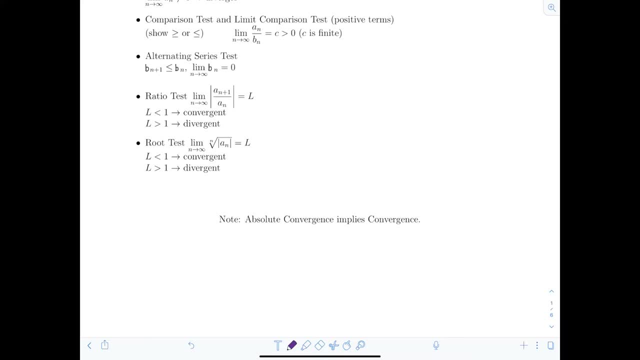 a different test And then root test: very similar limit, as n approaches infinity, of the nth root, of the absolute value of a n. If that comes out to be some value that's less than 1,, your series is convergent, and if it's greater than 1, divergent And the 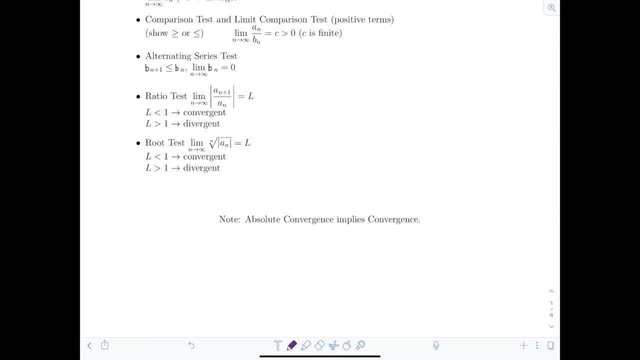 last two, the ratio and the root, automatically test for absolute convergence. And remember, absolute convergence implies convergence. Absolute convergence is a stronger type of convergence. So here we go, and as I work through the examples, I'll explain why I chose what test to apply. all right, 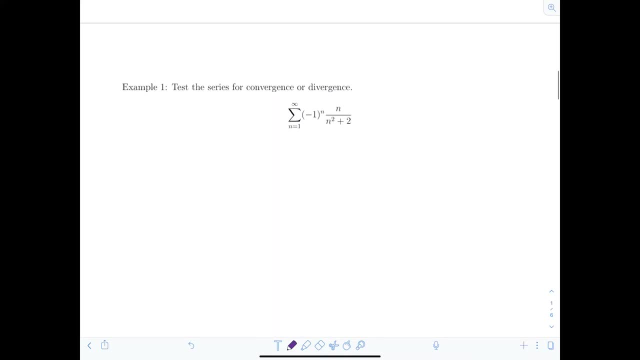 Because that's probably going to be the most difficult part. So example 1, test the series for convergence or divergence. So right away I notice it's alternating right. You see that negative 1 to the n, So it seems like a good time. 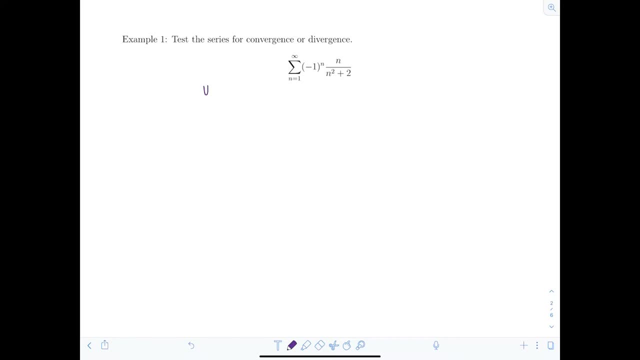 to use the alternating series test Use AST. So let's check the conditions, okay, Remember, Bn is the absolute value of An, so you just get rid of that alternating part, the negative 1 to the n, and I'm left with n over n squared plus 2.. Okay, 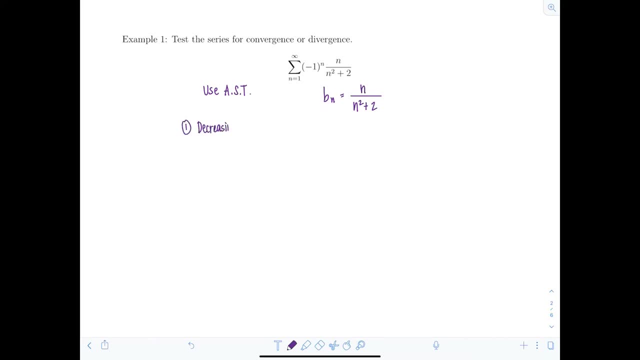 so first I want to check: is it D-card, D-card, D-card, Increasing? Okay, and the easiest way to check is by using the derivative. So first I have to find a fun- define a function. So let f of x equal x over x. 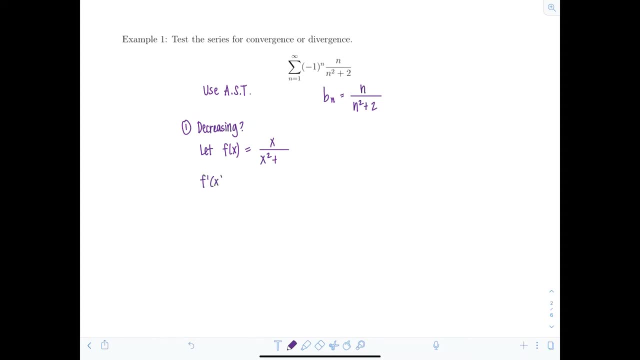 squared plus 2, and then f prime of x is going to equal- now I have to use the quotient rule, So I'm going to have x squared plus 2 times 1 minus x times 2x over x squared plus 2.. 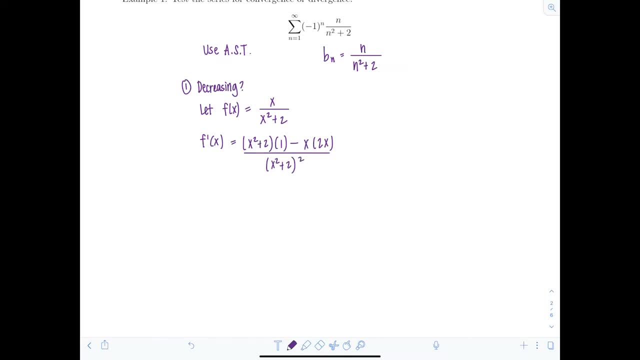 squared. Good, And then if I distribute and simplify in the numerator, I'm going to have negative x squared plus 2 over x squared plus 2 squared. Well, what can I say about this derivative? Well, I know the denominator is always going to be positive. and then the 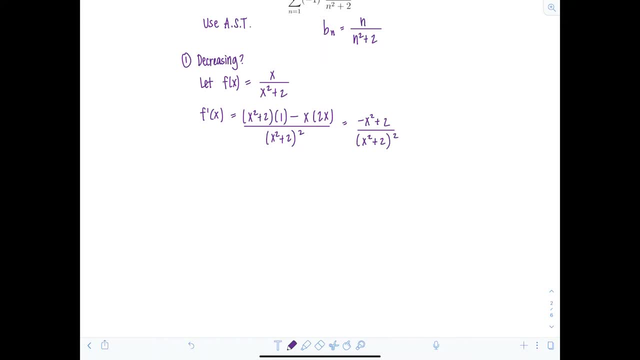 numerator is going to be negative just as long as x is greater than or equal to 2, right, So we could say that this is going to be positive and then the numerator is going to be negative. So this derivative is negative for x's greater than or equal to 2, which means that b sub n is: 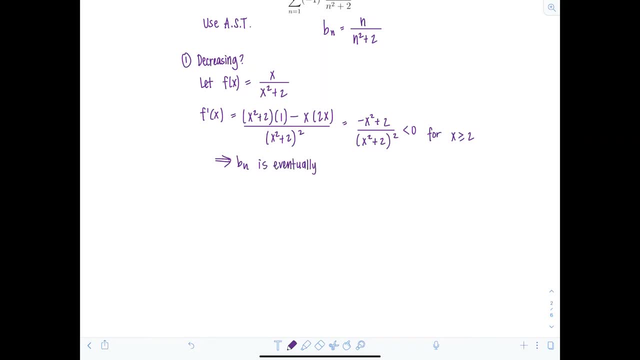 eventually decreasing. That's good enough for us. Okay then condition two. I want to check the limit as n approaches infinity of b sub n. So that's going to be the limit as n approaches infinity of n over n squared plus 2.. Now, remember to take this limit. I'm going to multiply numerator and. 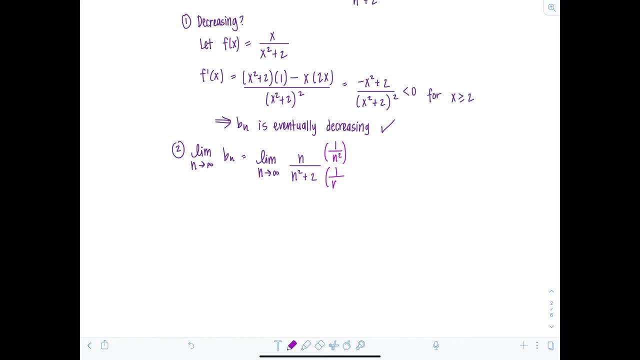 denominator by 1 over n squared, Always use the highest power of the variable from the denominator, And then this is going to equal the limit, as n approaches infinity, of 1 over n over 1 plus 2 over n squared. All right, And then, as I take this, 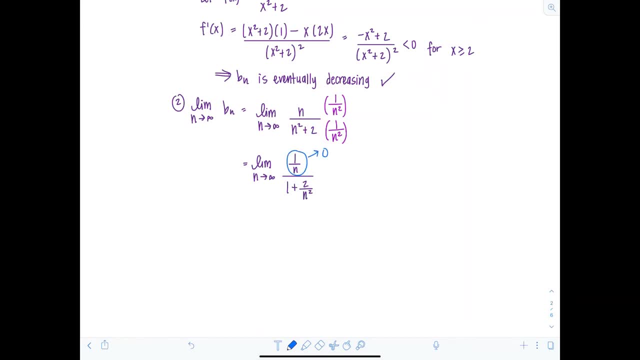 limit: 1 over n, that's going to approach 0.. 2 over n, squared, that goes to 0.. So now I'm left with 0 over 1, which is 0.. Yay, So both conditions are satisfied. What does this mean? Well, this implies: 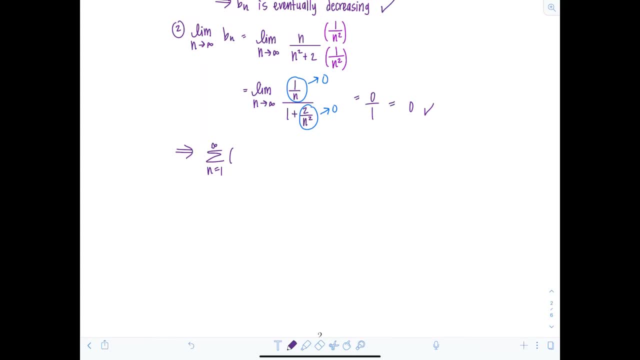 that the sum n equals 1 to infinity. always rewrite the original negative 1 to the n times n over n squared plus 2 converges. So we are going to print it out And then we is going to help us to get the reduced. 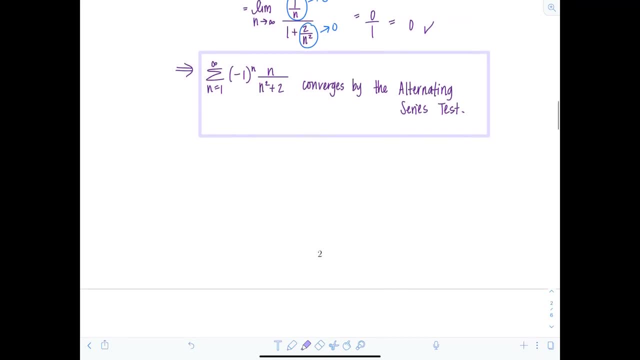 length- which is a nice thing- By the alternating series test. I'm going to look at it again Now. let's see if I can反akelify something to the expression. if such terms were real, forever, This is really nice. I'm going to daddy there. Let's test the series for convergence. 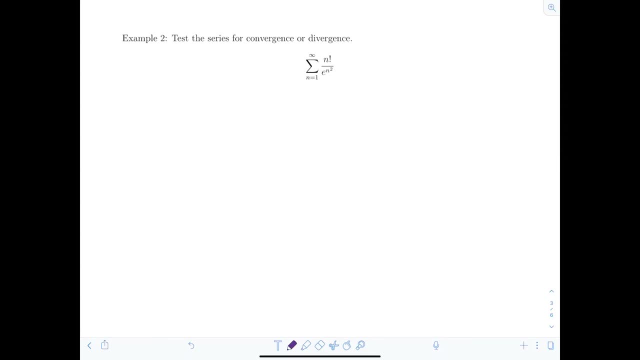 or divergence. So first we're going to do the n-inverting by 1 plus n, so n approaches infinity of n to the negative 0 over n squared. then outwards, The general expression would be n plus d raised n factorial over e to the n squared The majority of the time. if you see the 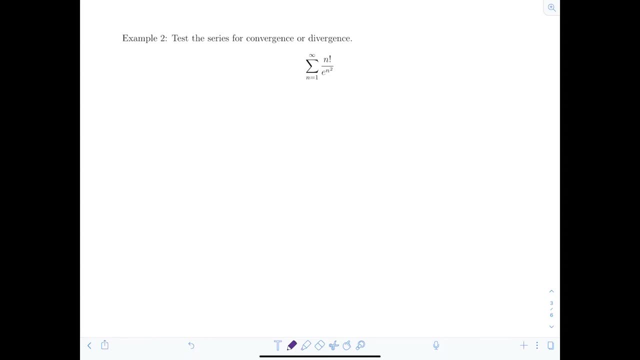 factorial sign somewhere in the terms of your series. it is time to use the ratio test, because when you have that ratio of a sub n plus 1 over a sub n and you have factorials, it makes for a beautiful cancellation, Okay. so remember that Ratio. 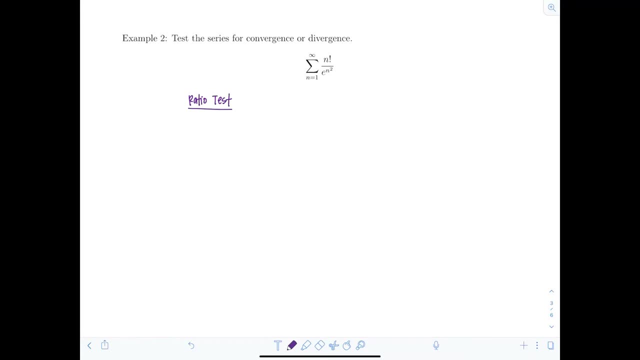 test. So we have the limit. as n approaches infinity, I'm going to have the ratio, absolute value of it, of a sub n plus 1 over a sub n. Okay, so this is going to be the limit. as n approaches infinity, I have the absolute value: a sub. 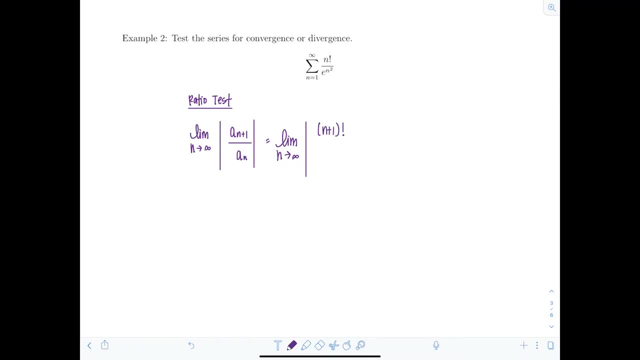 n plus 1 is going to be n plus 1 factorial Over e to the n plus 1 squared. Okay, and then if I'm dividing by a sub n, I'm just going to multiply by its reciprocal: e to the n squared over n factorial. 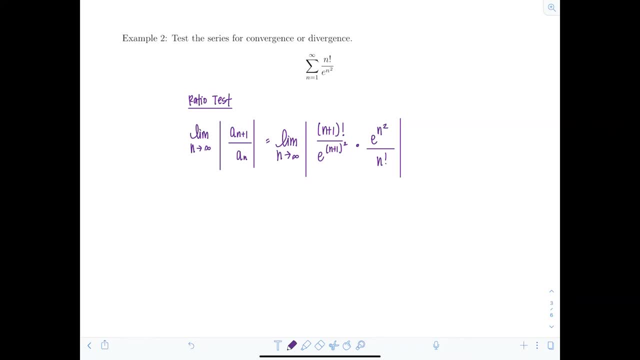 Alright, now, looking here, nothing's negative. I don't need the absolute value anymore. And then I'm going to start breaking up the factorials and everything so I can expand and start canceling. So I have the limit as infinity. And then I'm going to start breaking up the factorials and 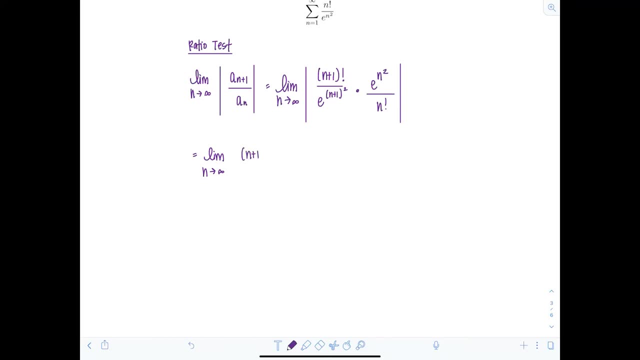 everything so I can expand and start canceling. So I have the limit as n approaches infinity. So n plus 1 factorial. for sure, I want to rewrite that as n plus 1 times n factorial. e to the n plus 1 squared. I'll write that as e to the n squared plus 2n plus 1, right. 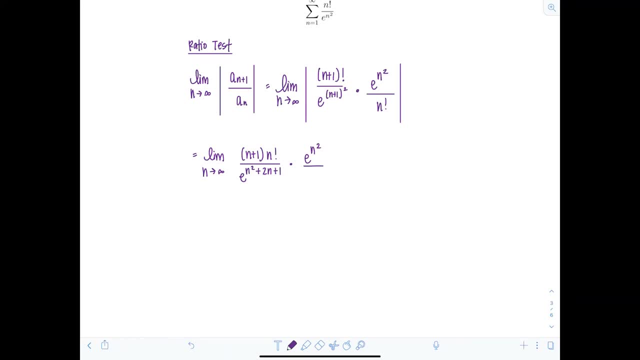 Times. and then I'm just going to leave this e to the n squared over n factorial. Okay, well, right away I notice I can cancel out the n factorial, so that's good. And then I want to break up this e to the n? squared. 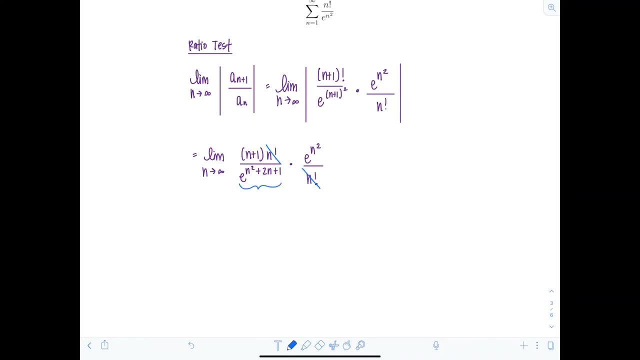 With this term here. So remember your rules of exponents. I can write e to the n squared plus 2n plus 1 as e to the n squared times, e to the 2n plus 1, right, Because you're adding your exponents when you're multiplying like that. So I'm just going to cancel out the n squared here with the entire e to the n squared in the numerator, And then now I'm left with the limit. 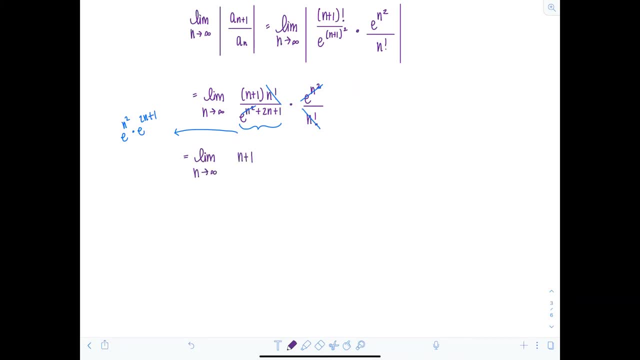 As n approaches infinity, I have n plus 1 still in the numerator and then e to the 2n plus 1 in the denominator. Okay, so how do we evaluate this limit? Well, the numerator is approaching infinity as n goes to infinity and the denominator is approaching infinity. 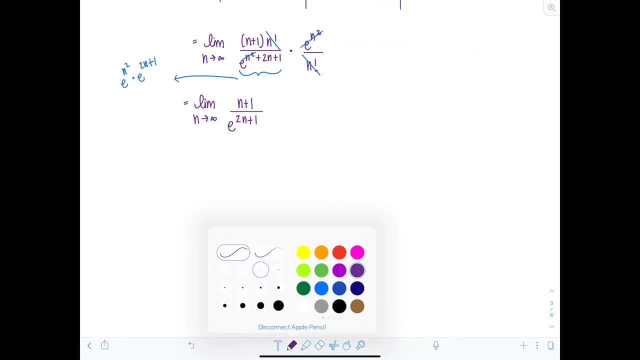 So we have an indeterminate form of the type infinity over infinity. So it's time to use L'Hopital's rule. but remember, you can only apply L'Hopital's rule to a function. So I'm going to let f of x equal x plus 1 over e to the 2x plus 1.. 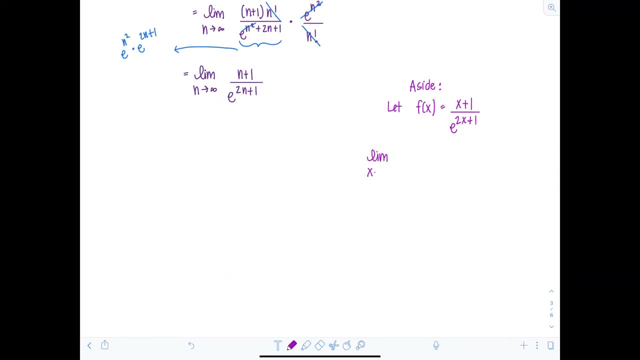 And then we're going to consider the limit, as x approaches infinity, of x plus 1 over e to the 2x plus 1.. And then this is the limit, indeterminate form of the type: infinity over infinity. So I'm going to use L'Hopital's rule to a function. 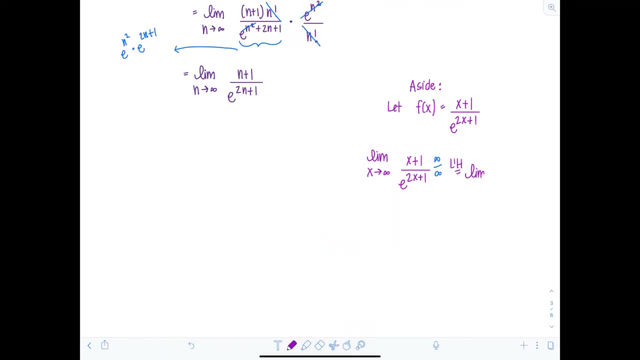 So I'm going to apply L'Hopital's rule. Now I have the limit. as x approaches, infinity Derivative of the numerator is going to be 1 over derivative of e to the 2x plus 1 is 2 e to the 2x plus 1.. 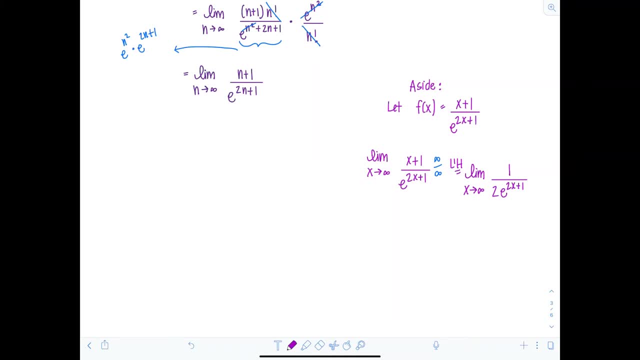 And as x approaches infinity the denominator is going to get very large. I have a constant in the numerator, so this limit is 0.. So now I know this limit here as n approaches infinity of n plus 1.. So I'm going to say l plus 1 over e to the 2x plus 1.. 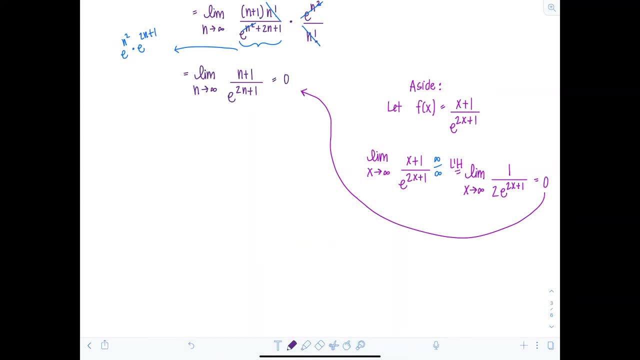 That's also going to be 0.. And then, don't forget, since we're using the ratio test, I always want to compare this to 1.. So 0 is less than 1.. What does that tell me? Well, this tells me that my original series, the sum- n equals 1 to infinity, of n factorial over e to the n squared, is convergent. 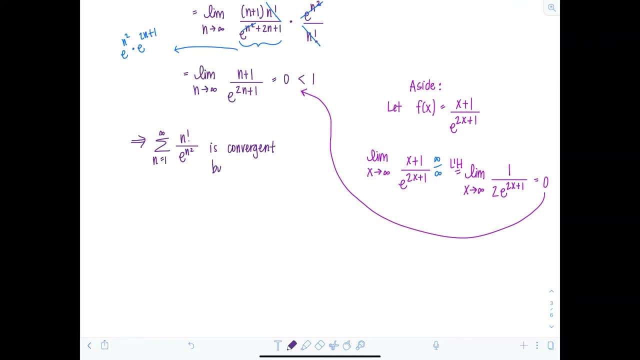 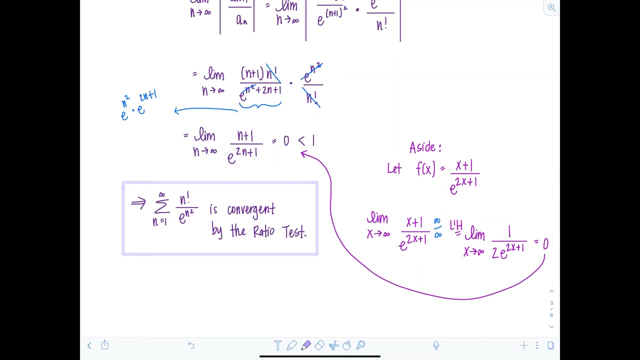 by the ratio, the ratio test. okay. so just as a note, if you're gonna apply L'Hopital's rule to take a limit in that way so you don't break your train of thought, you can do it off to the side and it's appropriate to write: this is being computed aside, do? 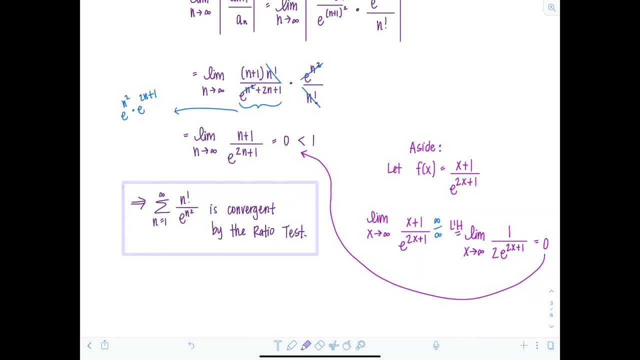 all your proper notation and limit-taking there, and then you can substitute the result in: okay, this would be a full credit answer. very nice, let's look at another example. that's always a fun test, don't you think so? example three test the series for convergence or divergence, and we have 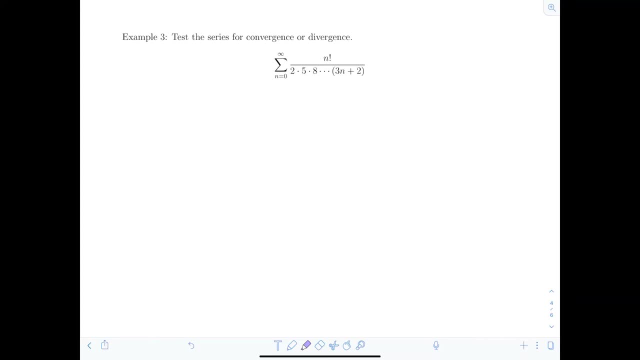 the sum, and equals zero to infinity, of n factorial over. and this is an interesting product. here we have two times five times eight, up until three n-minutes plus two, so you're multiplying. it's not gonna involve factorial notation because you're jumping by threes, but we're just gonna follow the pattern here and again. 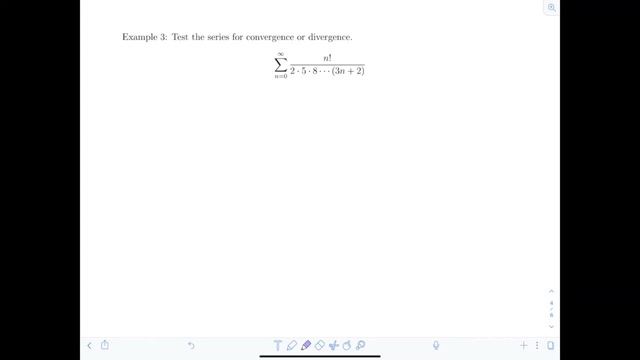 I'm gonna use the ratio test because of that factorial. it's gonna cause for some lovely cancellation, so we're using the ratio test. okay, we're gonna look at the limit, as n approaches infinity, of the absolute value of a sub n plus one over a seven. 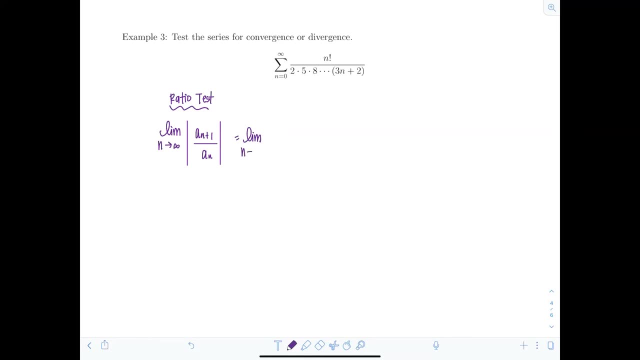 okay. so this is gonna be the limit and approaches infinity. I have absolute value and plus one factorial in the numerator over now be careful here. so this is two times five times eight, up until three n plus two. but if I substitute in n plus one here, I'm gonna have to distribute that three, so it's. 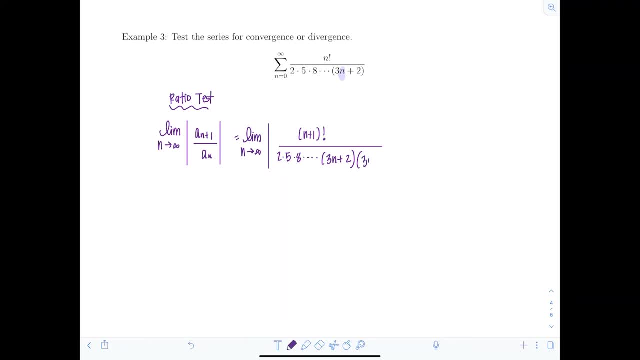 gonna give me three n plus three, and then I have plus two, so this is three n plus five, right? so this whole thing here, this is a sub n plus one, and then I'm gonna divide by a sub n, so I'm gonna multiply by the reciprocal, which is two times five. 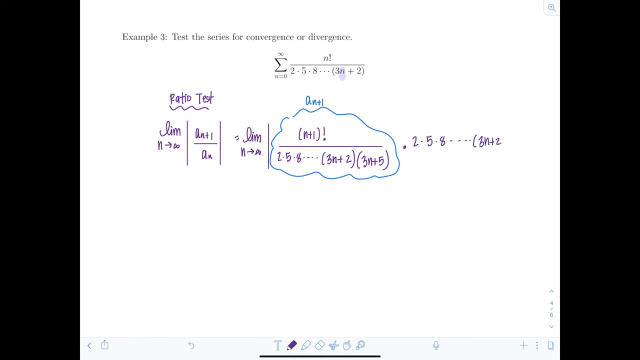 times eight up until only three. n plus two over and factorial. all right, let's look at subtree法, root of just simply dt, No limitز. All right, looks good. Now we can start canceling. So remember this: n plus one factorial is n plus one times n factorial. 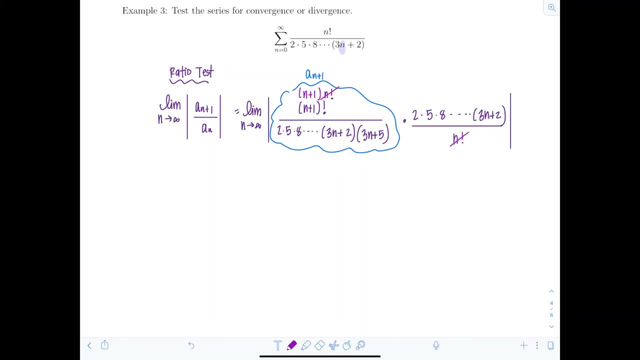 So I can cancel out that n factorial with the n factorial in the denominator, And then this whole numerator cancels out with almost everything in the denominator. here The only survivor is three n plus five. Okay, so I've got an n plus one in the numerator left over. 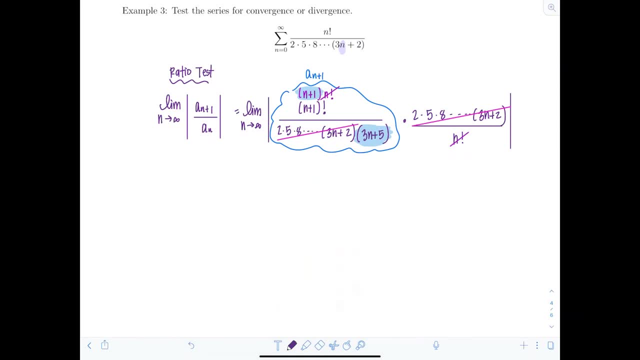 and then three, n plus five in the denominator. that's it, And I don't need absolute value. Nothing's negative. So I have the limit, as n approaches infinity, of n plus one over three, n plus five, And then the degree of the numerator. 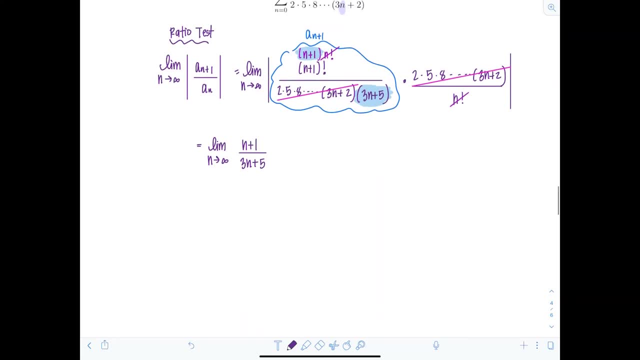 equals the degree of the denominator. So I can just take the ratio of the leading coefficients as n approaches infinity, which is gonna be one third. And then what do I need to say? Don't forget, one third is less than one, which tells me that the sum n equals zero to infinity. 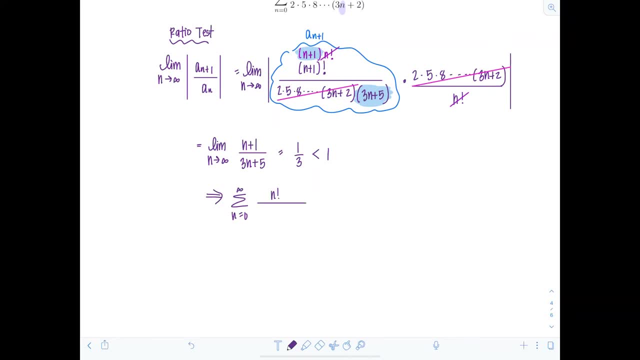 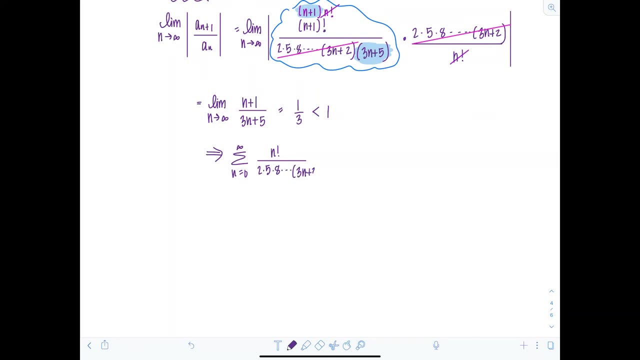 of n. factorial over. you have to write it out, Don't just write a n and be lazy. okay, And factorial over. two times, five times eight, up until three. n plus two converges by the ratio test. Okay, That looks nice. 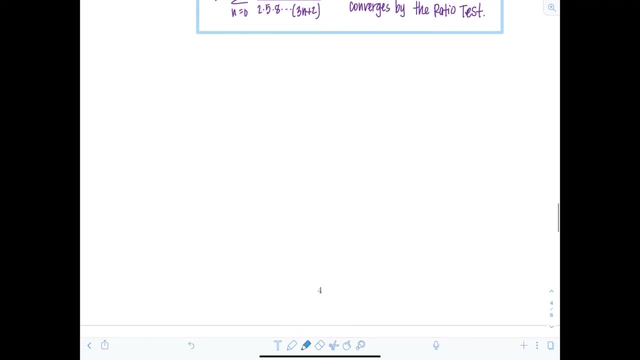 Don't worry, all the rest won't be ratio test. Here we go. We're gonna spice things up a little bit with our next example. So test the series for convergence or divergence. We have the sum n equals one to infinity of tangent of one over n. 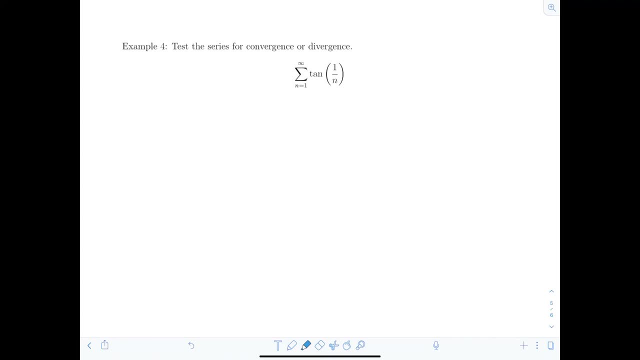 Okay, first things first, do a quick test for divergence in your head. So just check: are the terms going to zero? So as n approaches infinity, one over n is gonna approach zero, And I know tangent of zero is zero. So test for divergence inconclusive. 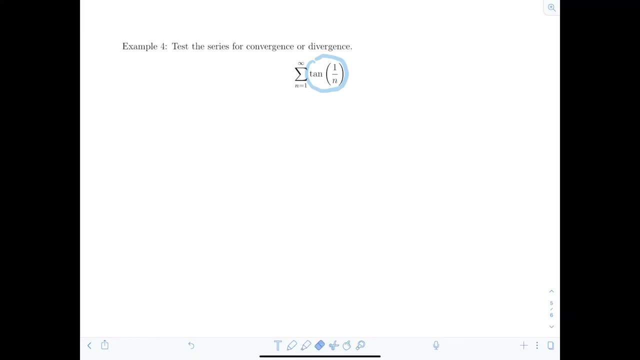 I don't know what's gonna happen. What other tests do I have? Ratio test, root test- they don't sound nice. Alternating series test is not appropriate now. Integrating tangent of one over x does not sound pretty, So I'm gonna kind of make light of the fact. 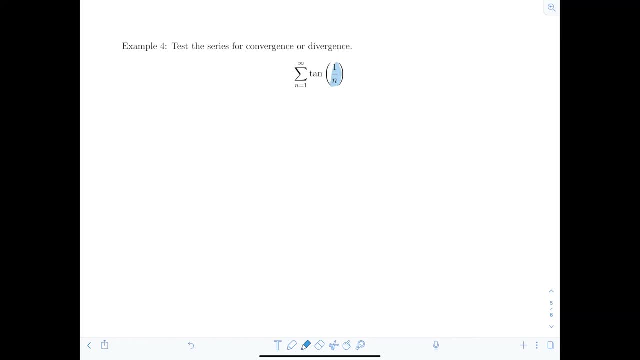 that there's this one over n appearing here and see if I can do some sort of limit comparison test. Okay, I'm not gonna try direct comparison because the tangent's gonna make things too difficult, But we're just gonna play around with the limit comparison test. 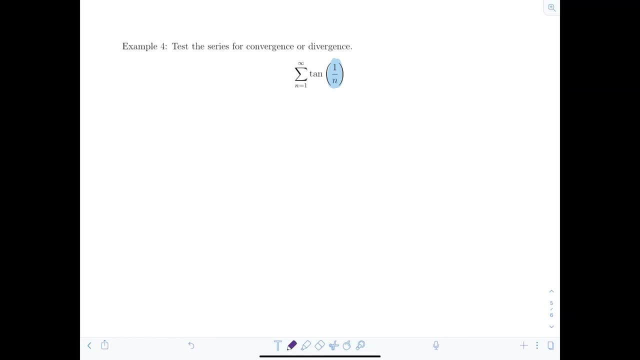 see if things work themselves out. So remember, if we're gonna use the limit comparison test, I have to identify first what I wanna compare it to. So I'm gonna consider b sub n, which is one over n, And I know that the sum n equals one to infinity. 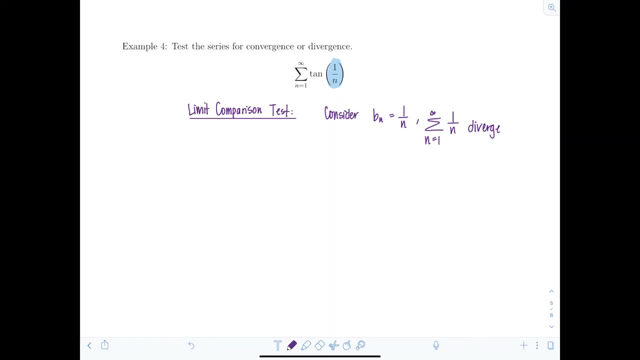 of b sub n diverges. Why is that the case? Because it's the harmonic series, Not really All right. so now I'm gonna look at the limit, as n approaches infinity, of a sub n over b sub n, And this is gonna be the limit as n approaches infinity. 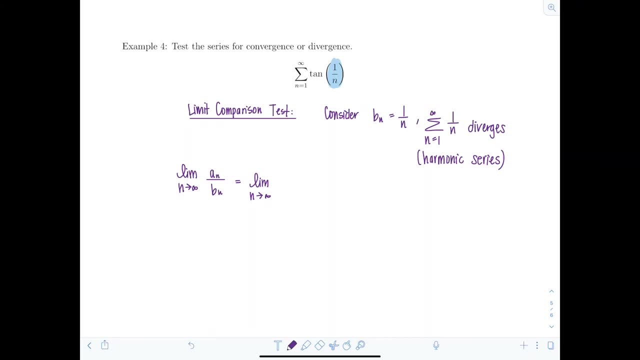 So a sub n, remember that's the terms of our series, So that's tangent of one over n over one over n. Okay, So now we have an indeterminate form of the type 0 over 0, right, Because as n approaches infinity, numerator is going to 0, denominator is going to 0.. 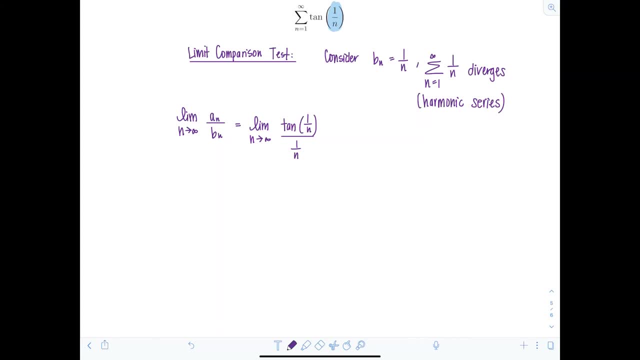 So you could redefine a function and you could use L'Hopital's rule. But we've done that plenty of times, So I want to show you a little bit different of a way to evaluate this limit. okay, First I'm going to say: let theta equal 1 over n. 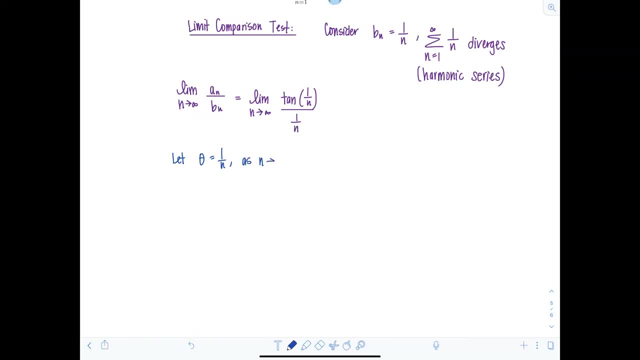 And we know, as n approaches infinity, this means theta approaches 0, okay, And also recall from early in your calculus career that the limit as theta approaches 0 of sine theta over theta is equal to 1.. Yes, you can confirm that using L'Hopital's rule, but you learned this limit long before then. 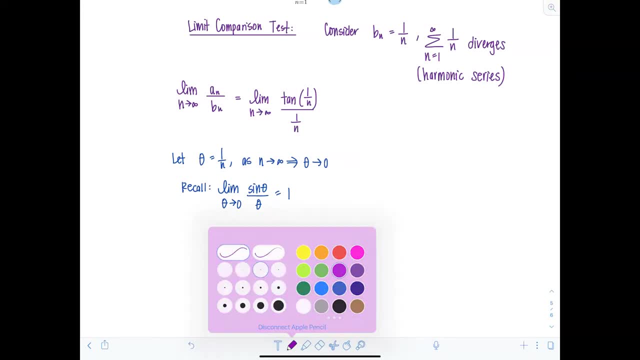 So I'm going to actually rewrite this limit here In terms of theta now. So I'm going to have the limit: instead of, as n approaches infinity, I'm going to use theta approaches 0. And then I'm going to have tangent of theta over theta. 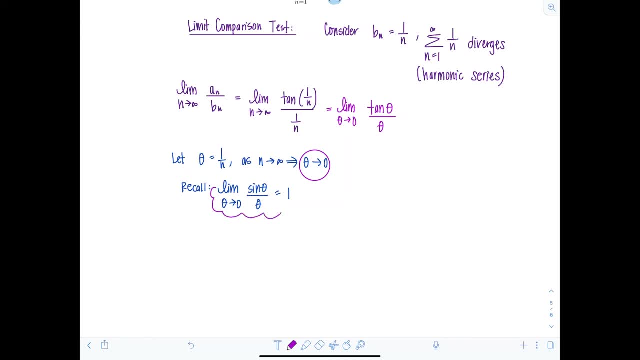 And now I can rewrite tangent in terms of sine and cosine to make use of this fact here. So I can write this as the limit as theta approaches 0 of sine theta over cosine. But I'm going to break it up a little bit. 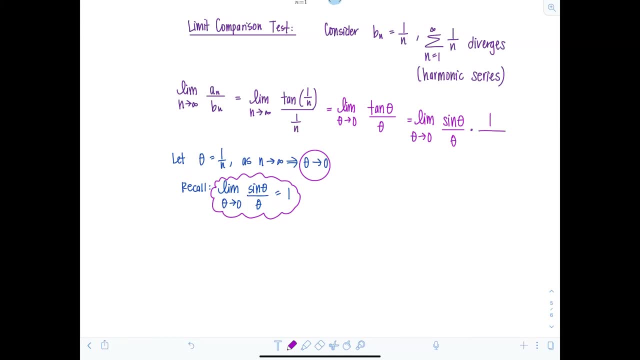 So I'm going to write sine theta over theta times 1 over cosine theta right. So here's my tangent, but I split it up in such a way because now I can say, ooh, sine theta over theta. this approaches 1, right. 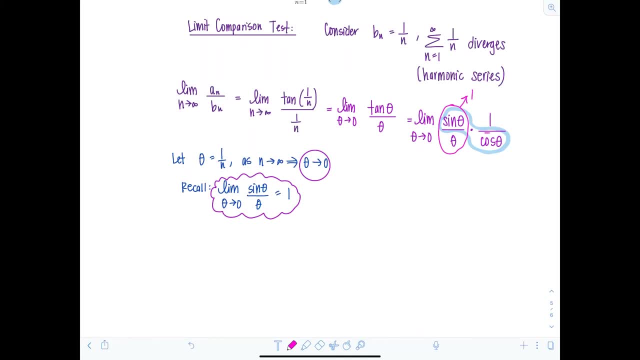 As theta goes to 0. And then as theta approaches 0,, cosine of 0 is just 1.. So this limit is actually equal to 1 times 1,, which is 1.. Now don't get confused, This is limit comparison test. 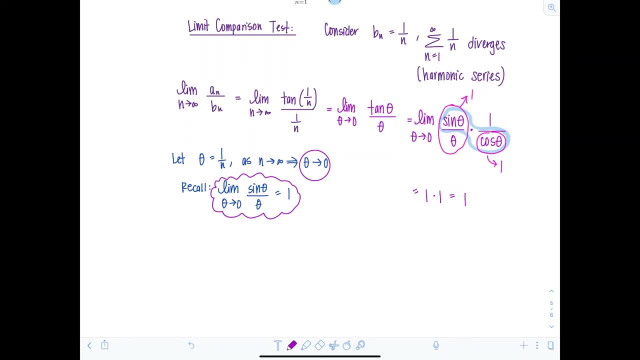 So what do I care about when I take this limit? That it's not negative, it's not 0. So how do I write that out? I just say this is greater than 0. So it's finite, right? You can't have an infinite limit. 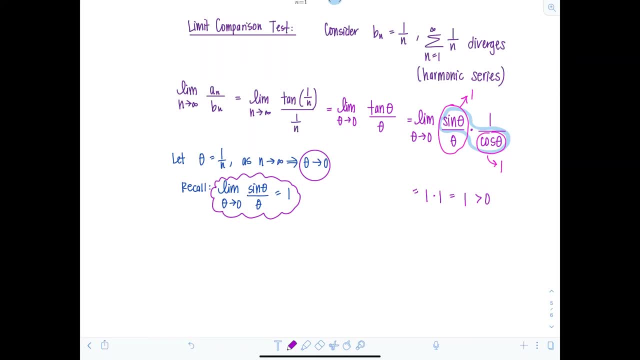 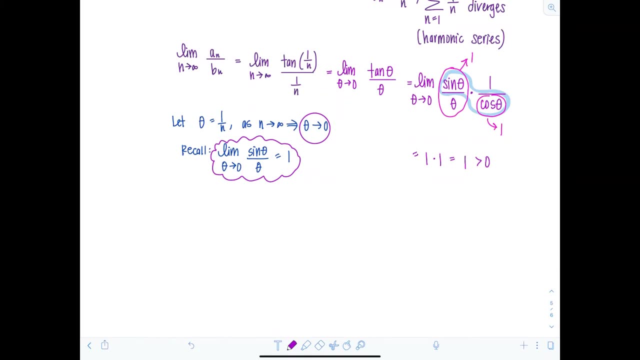 That's inconclusive. You can't have 0.. That's inconclusive. So what does that tell me? When you get this constant, then that means that the series that you're investigating behaves the same as the one you were comparing it to. 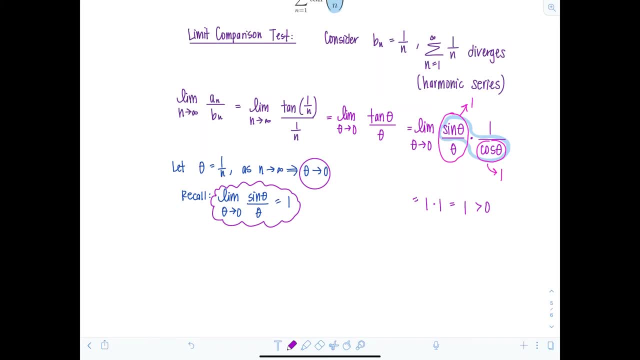 And so since the harmonic series diverges, that means our series diverges as well. okay, So when you get that finite constant from the limit comparison test, that means both series behave the same way. They either both converge or they both diverge. 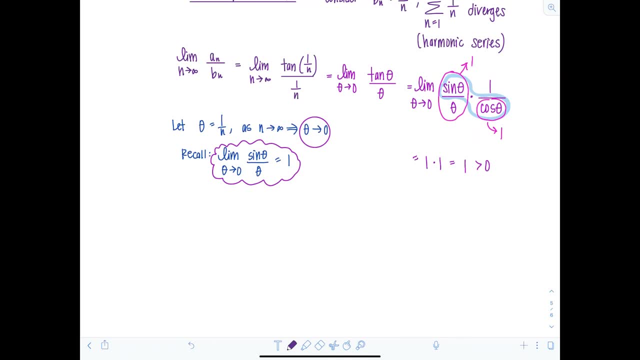 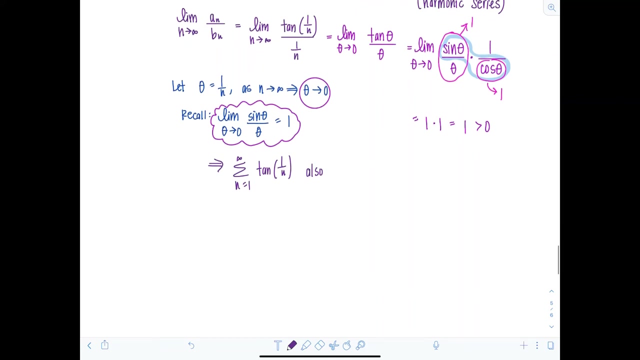 It doesn't matter what the value is either. It could be 1, 1 fourth 100. It doesn't matter. So this tells me that the sum n equals 1 to infinity of tangent of 1 over n also diverges by the limit comparison test. 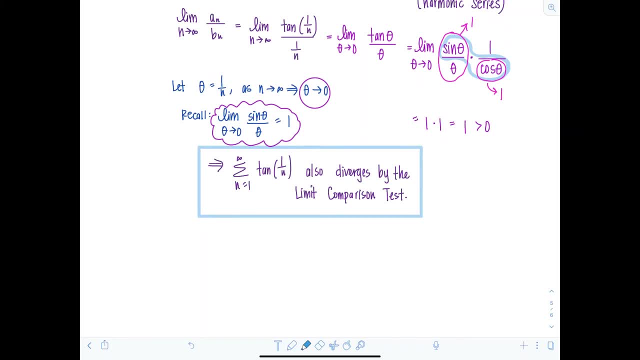 All right, And again, you could have done that limit, redefining a function and using L'Hopital's rule, if you like. Just one more time? All right, All right, All right. I just wanted to do something a little different. 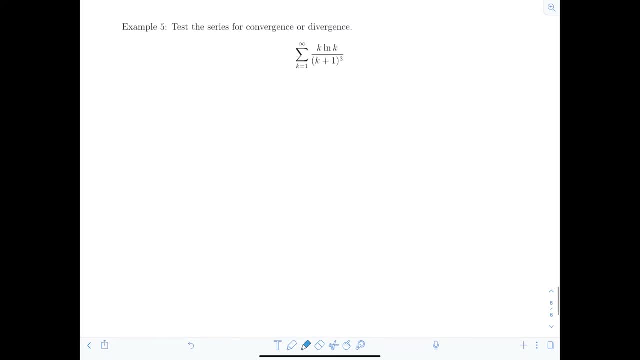 Okay. Last example, taking it to the next level, test the series for convergence or divergence. Okay, First things first. these terms look scary, right? I see a natural log. Ooh, maybe it's going to be time to integrate. 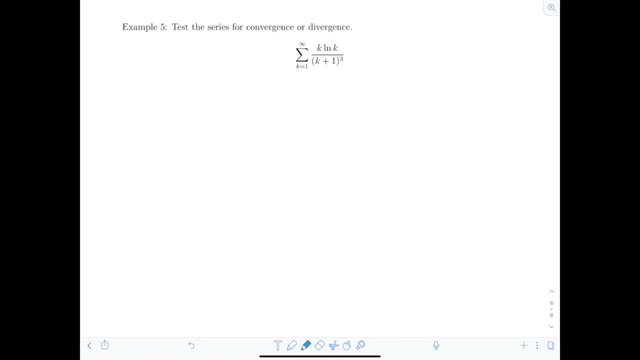 We're feeling an integral test, But the way things are written I really don't want to integrate this expression. It looks kind of scary, So I'm going to use action. It's actually a combination of two tests. I'm going to first simplify this expression. 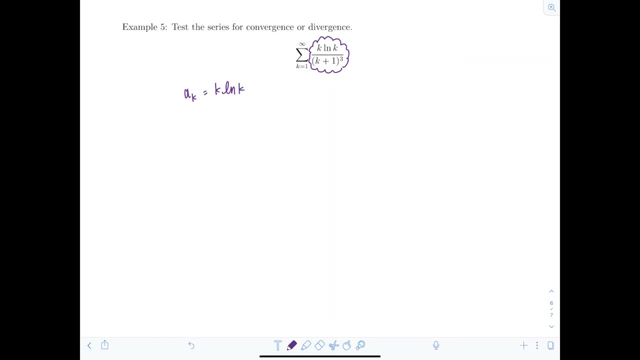 So a sub k is k times natural log of k over k plus 1 cubed, And I'm going to use the direct comparison test and the integral test in order to deal with this. I don't want to integrate a k directly. I'm going to integrate another set of terms. 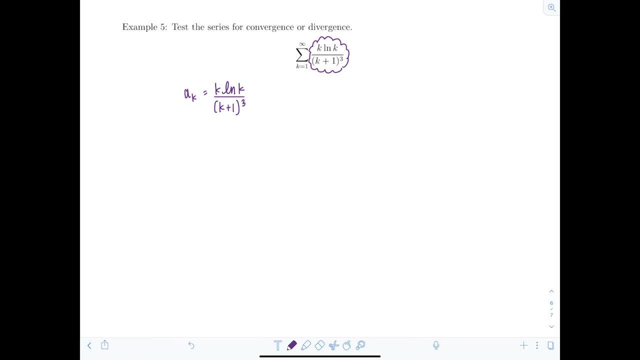 That way I can. All right, I'm going to work with an easier integral, basically. Okay, So I can say a sub k. the terms here are less than k times natural log of k over just k cubed right. 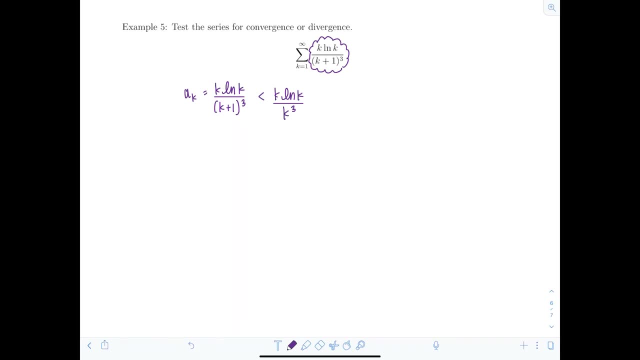 instead of k plus 1 cubed, because now this denominator right is larger, So the whole expression would be smaller. And then the reason I did this was: look, look, I can cancel out this k. and now this is the k squared. 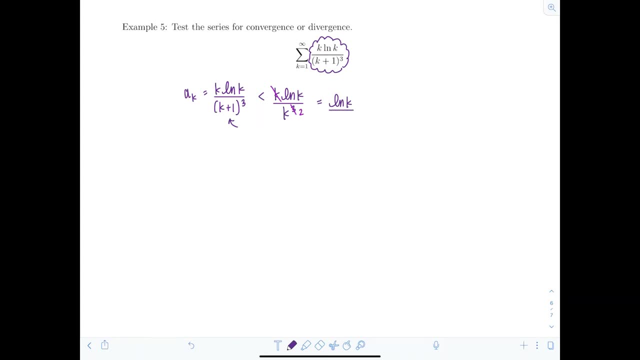 Why does that make me happy? Well, because I can integrate this ln of k over k squared a lot more easily than I could integrate the original terms a sub k. So I want to apply the integral text. Remember I have three conditions to check. 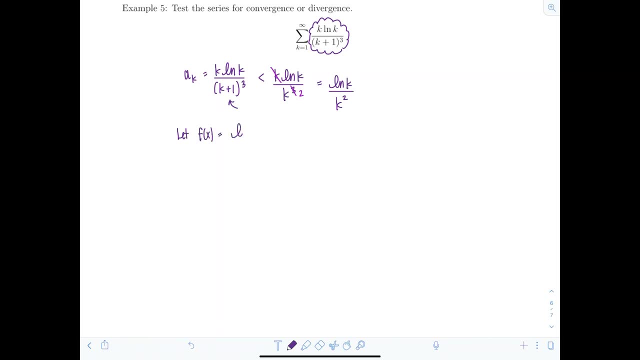 So I'm going to let f of x equal natural log of x over x squared. Okay, Are the terms positive? Well, on 1 to infinity, they're eventually going to be positive, right? All right, Let's see if they're going to be positive. Okay, All right. So now let's try this. If x is less thanела, then is that not going to make a difference? You know whether it's positive or positive. that can't be positive, Okay, But I'm going to find that. 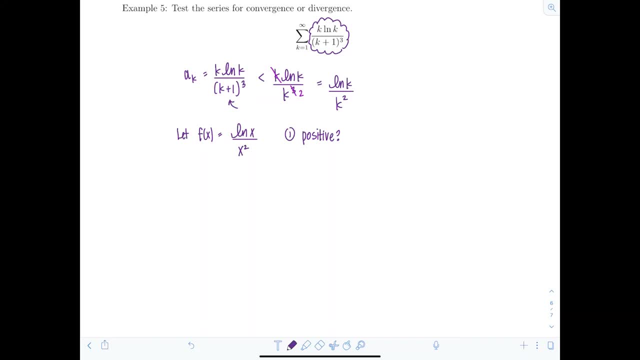 There you go. All right, ln is 0 when x is 1, but then after 2, then we're going to be okay, So it's eventually fine. Is it going to be continuous on 1 to infinity? Well, what's the domain here? 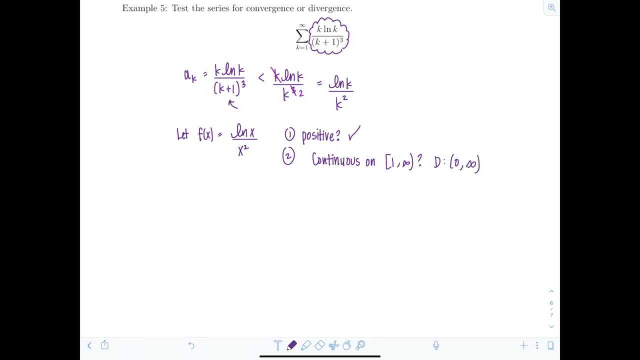 The domain is from 0 to infinity, not including 0, which is a subset of 1 to infinity. So we're good to go. Or 1 to infinity is a subset of 0 to infinity, Excuse me. And then the last thing is: is it decreasing? 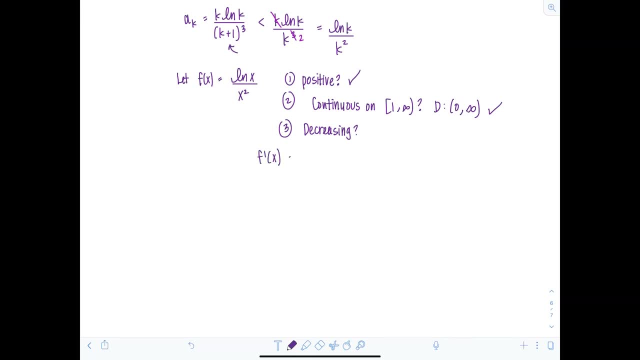 Well, let's take the derivative and see: So: f prime of x is going to be x squared times 1 over x minus natural log of x times 2x over x to the fourth. Okay, so I'm going to have x minus 2x, ln x, so I can factor out an x. 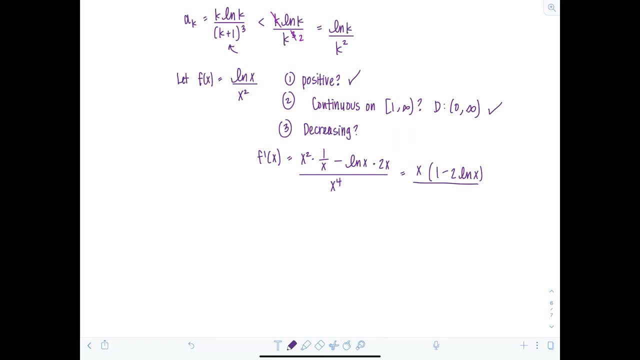 And then I have 1 minus 2 ln of x over x to the fourth, So I can write this as canceling out an x: 1 minus 2 ln of x over x cubed. Okay, well, remember, you're only substituting in values for x from 1 to infinity, right. 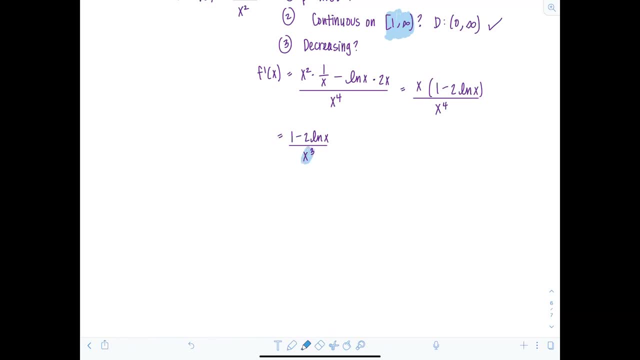 So the denominator is going to be positive. That's fine. What about 1 minus 2 ln of x? Well, as long as x is greater than rad e, that's going to be negative. So this is less than 0 for all. x is greater than rad e. 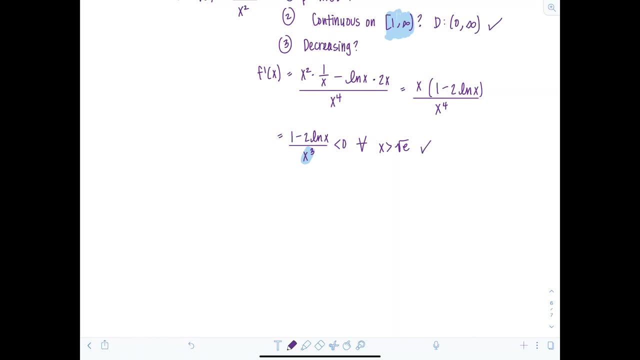 So that means the derivative is negative, which means it's eventually decreasing. So that means it's okay to apply the integral test. So let's go ahead and do that now. So I'm going to apply the integral test. So I'm going to integrate from 1 to infinity ln of x over x squared. 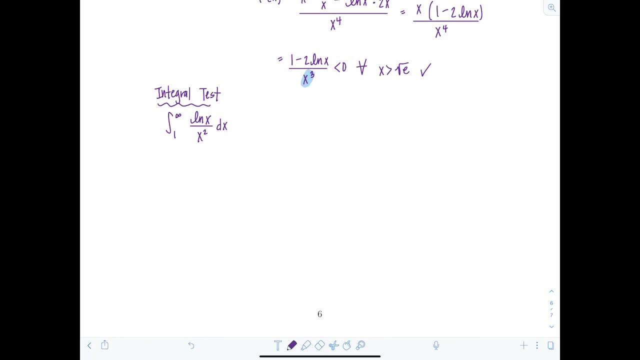 dx. right, Remember, this is not our original, the terms from our original series ak. This is something that is an upper bound for ak, So first thing I need to do is rewrite this as the limit as t approaches infinity, from 1 to t of ln of x over x squared dx. 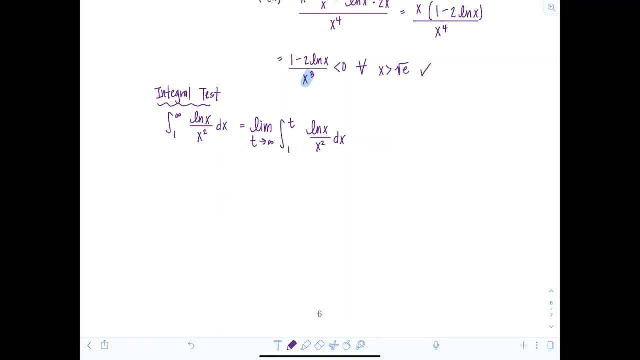 And then how do we anti-differentiate this thing? My goodness, it's time to use good old integration by parts. So if you just want to do this, you can do this. You just want to get the general anti-derivative off to the side. 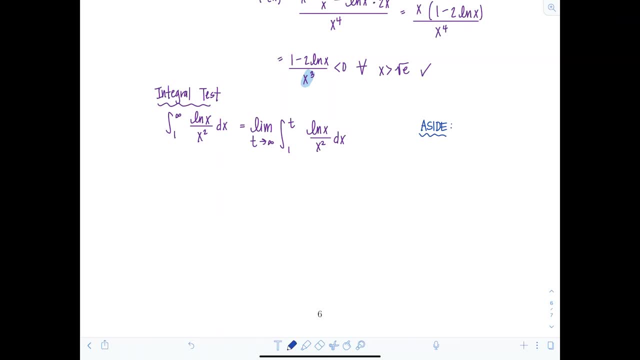 so you don't have to mess with the limit And the limits of integration. you can do that. So we're going to let u equal ln of x. dv is 1 over x squared dx, so x to the negative second dx. 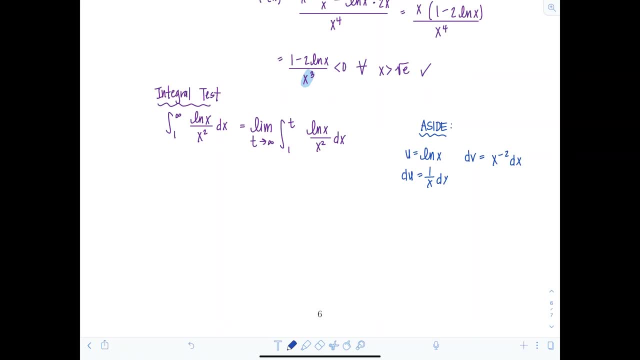 Then that means du is 1 over x, dx And v is negative, x to the negative first. Okay, so that integral ends up giving us negative ln of x over x. right, You take this product minus, so it'll turn into plus. 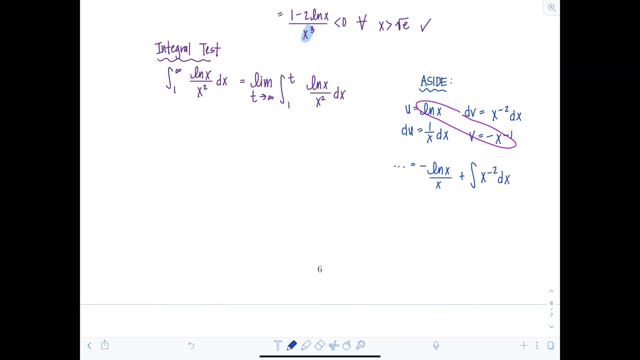 the integral of x to the negative second dx minus this product, And then this is going to give us negative ln of x over x minus 1 over x plus c. So then I can just substitute that in To my original limit here. So I have now the limit as t approaches infinity. 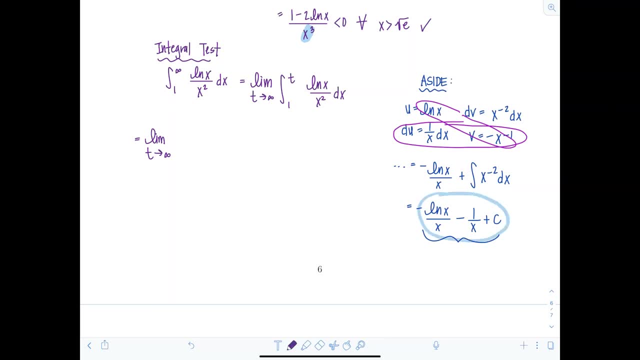 This whole expression is my anti-derivative. So now I have negative ln of x over x minus 1 over x, And then this is evaluated from 1 to t. Okay, you don't want to do your by parts within the limit. 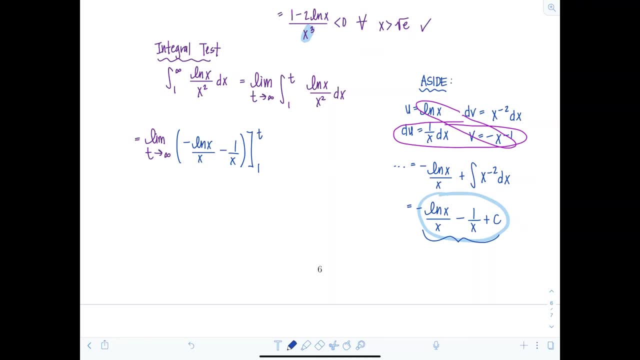 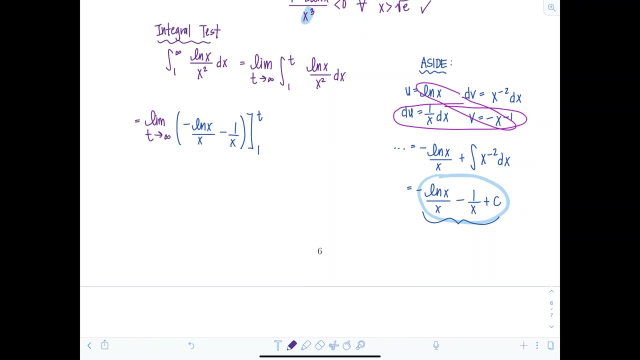 and then get sloppy. You want to do it with your limits of integration, So that's why I tend to do it off to the side. That way, I'm not having any notation errors. Okay, so back to this limit. Now we're going to evaluate it at its limits of integration. 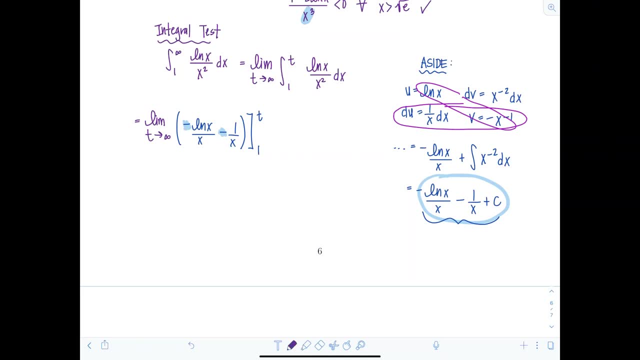 Notice here this negative. I can take that outside just to make things a little cleaner. So I have negative and then limit as t approaches infinity. Now I'm going to substitute in the upper limit t for x, So I'm going to have ln of t. 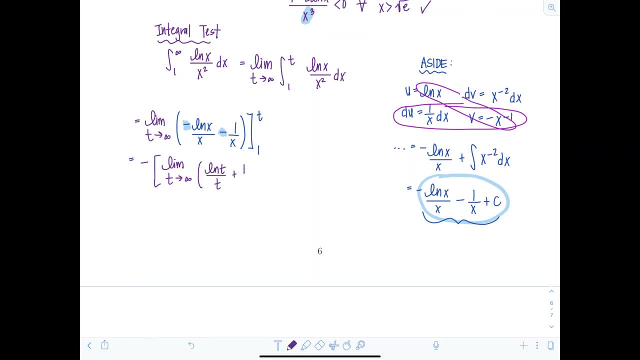 Over t plus 1 over t minus, and then the lower limit. now, Remember, the negative is outside. So we have ln of 1 over 1 plus 1 over 1, which is 1.. All right, good, Now let's go through term by term and evaluate this limit. 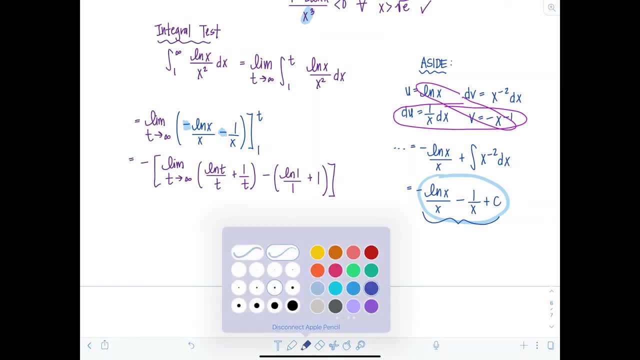 So, as t is approaching infinity, first thing I notice here is ln of t is approaching infinity. t is approaching infinity, So I have an indeterminate form of the type infinity over infinity. What does that mean? We need to apply L'Hopital's rule. 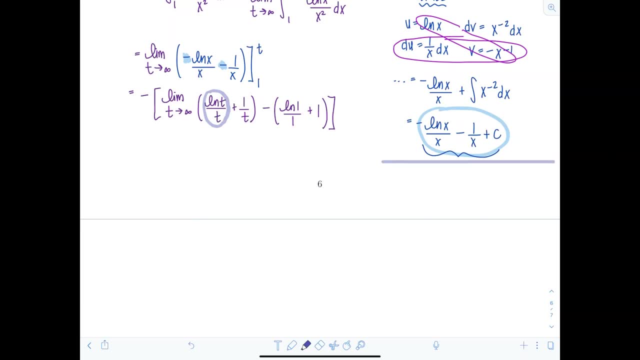 So we're going to do this work off to the side here, Let's put a little asterisk. So aside Again, we're going to look at the limit, as t approaches infinity, of ln, of t over t, And so we have indeterminate. 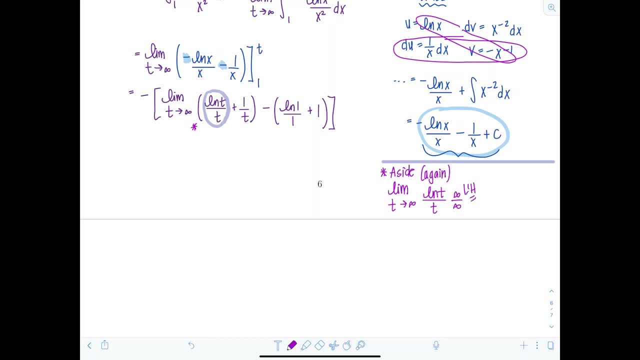 Form of the type infinity over infinity. So I'm going to apply L'Hopital's rule. I have the limit: as t approaches infinity, derivative of the numerator is going to be 1 over t, derivative of the denominator is just 1.. And as t approaches infinity, this limit is 0. 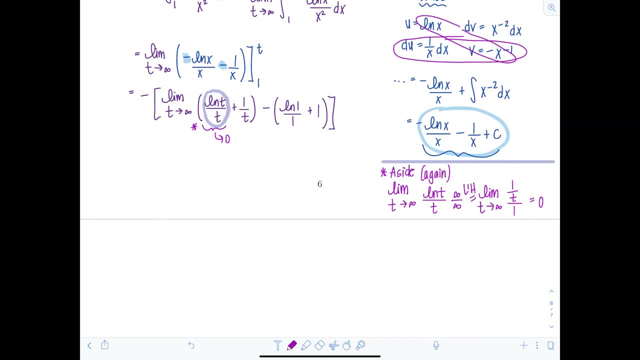 So now I can say ln of t over t, That terms going to approach 0.. As t approaches infinity, 1 over t, That's clearly going to 0.. Minus well, ln of 1, that's just 0.. 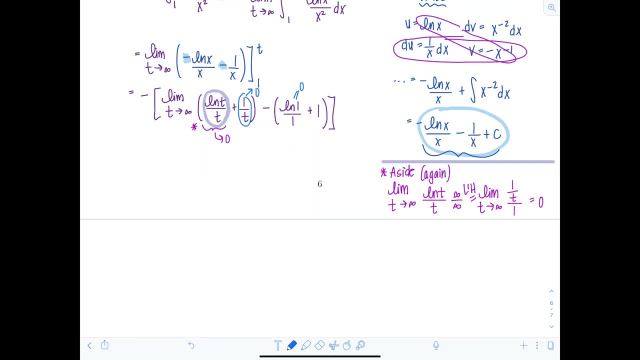 So that's done. And then the last term is a constant. So this 1 here is the only term that survives, And there's a negative here and the other negative sitting outside, So the result of this whole limit is going to be 1.. 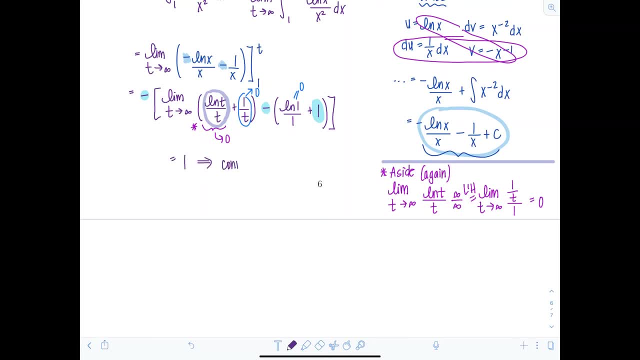 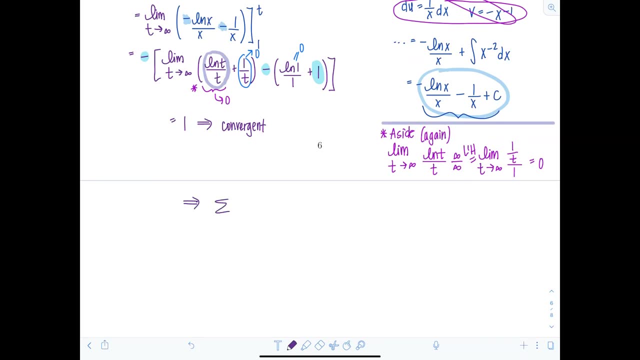 Which means that the improper integral is convergent. So what does that tell us? Well, first, this tells me that the, The sum k equals 1 to infinity of ln, of k over k squared, converges by the integral test. But remember, this is not the original series that we were testing for convergence or divergence. 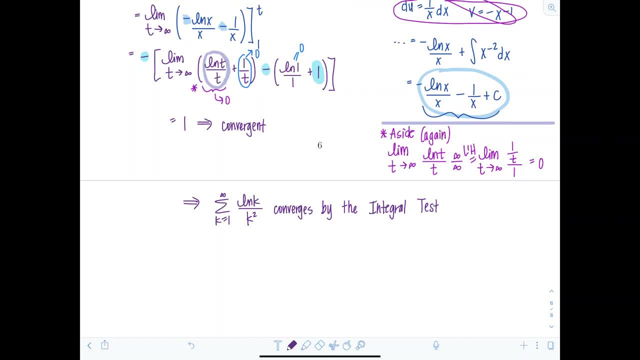 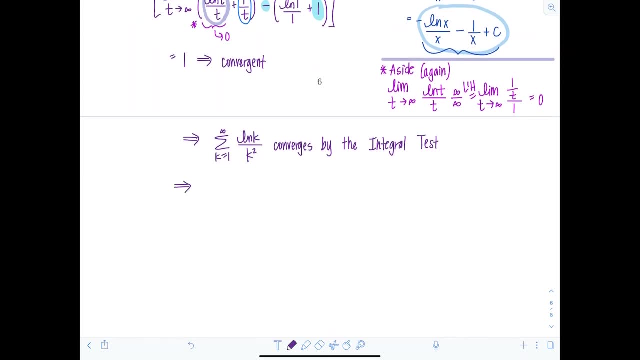 The terms of our series are smaller or bounded above by the Of this series which converges, And so, using direct comparison, Now I can say that my series converges, which is why we showed that inequality in the beginning. So now I can conclude that the sum k equals 1 to infinity of k times ln of k over k plus 1 cubed. 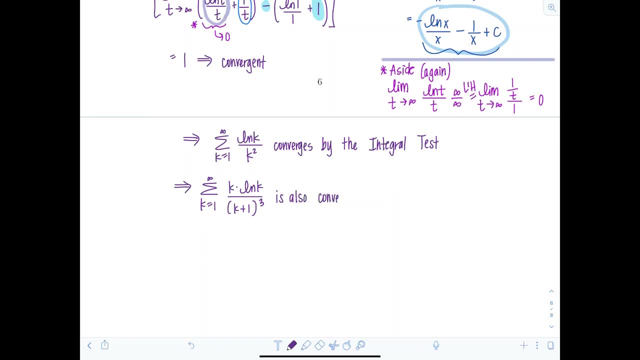 Is also convergent By the comparison test. Okay, and most of the time when we do the comparison test, the series which you compare it to, Typically you can just tell by looking or do a quick little check and state whether it's convergent or divergent. 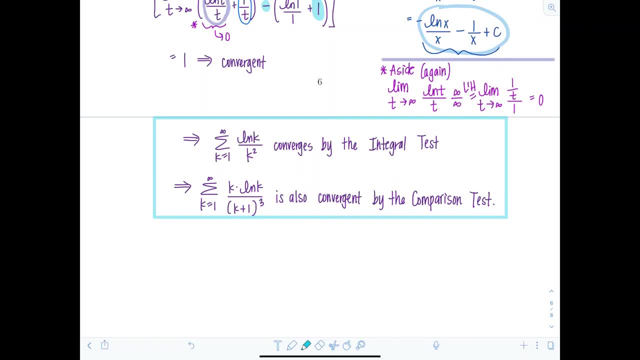 In this case, in order to establish convergence of this series here ln of k over k squared, We had to apply the integral test. So we had to do a combo of two tests here. So Make sure you pay attention to the details and the argument. 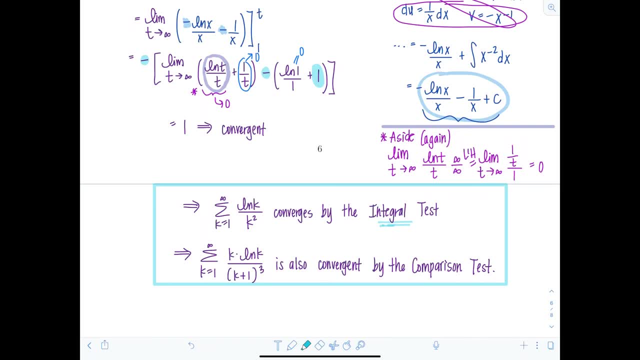 All right. If you have any questions or comments, feel free to leave them below and stay tuned for more videos.